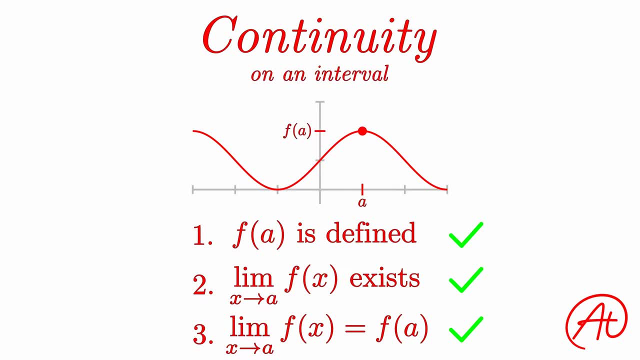 interval. In order for a function to be continuous on an interval, the function just needs to be continuous at every point, in the same way we just discussed, along the entire interval. Or another good way to think about it is if you can draw the function without picking. 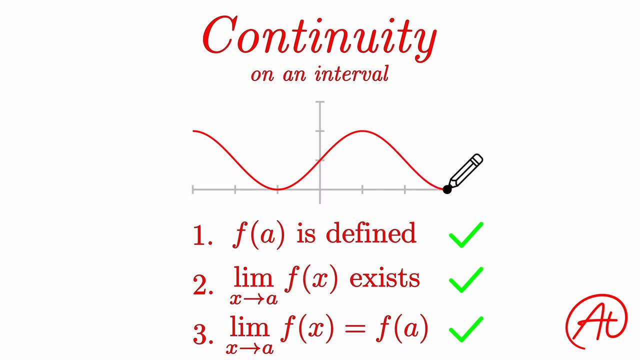 up your pencil, then it is continuous along that interval. So now, using this information, let's take a look at what causes some functions to be discontinuous. In this example, the function is not continuous because there is a hole right here with no other value for that x, so f is not defined for that point. 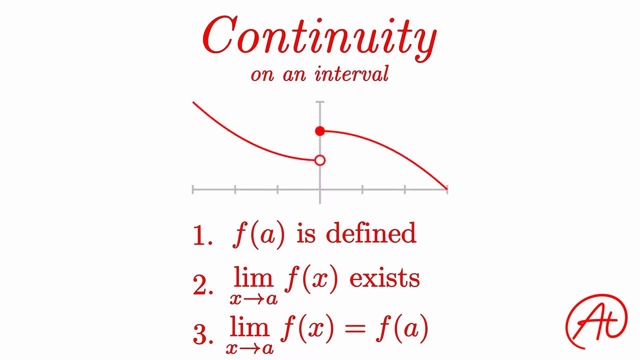 In this example there is another hole at x equals zero, but this time the function does have a value for this x. it's right here, so f is defined. However, for this example, the limit as x approaches zero from the left is this point, but the limit as x approaches. 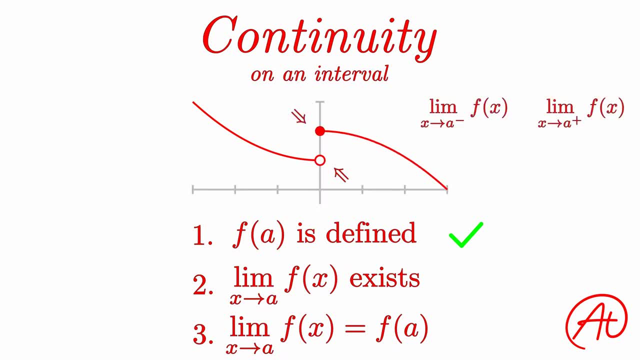 zero from the right is this point. so the two limits are not equal, making the overall limit as x approaches zero not exist. Now for this example. once again, f is defined where the hole in the function is. so we pass the first rule, This time the limit as x. 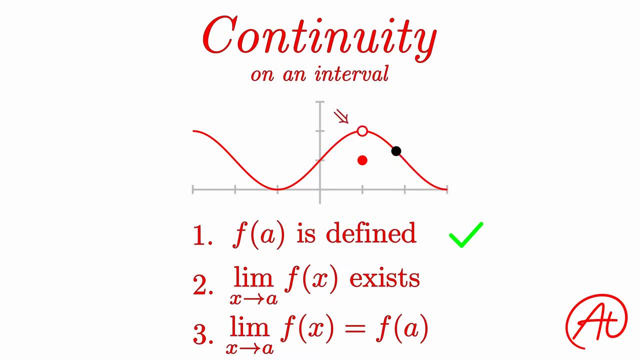 approaches a from the left is here, and the limit as x approaches a from the right is that same value. so the overall limit does exist. However, for this function, the overall value for the limit does not equal the value of f at that point, so this violates the third. 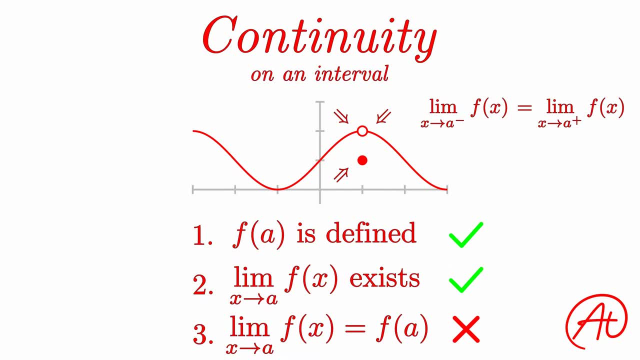 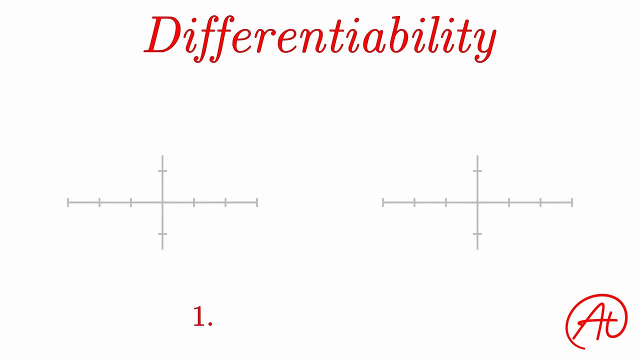 rule and makes the function discontinuous. Okay, now that we went over continuity, let's discuss differentiability. But first, if you're finding this video helpful so far, please smash those like and subscribe buttons to support us. Alright, just like we did for continuity, let's first talk about differentiability at 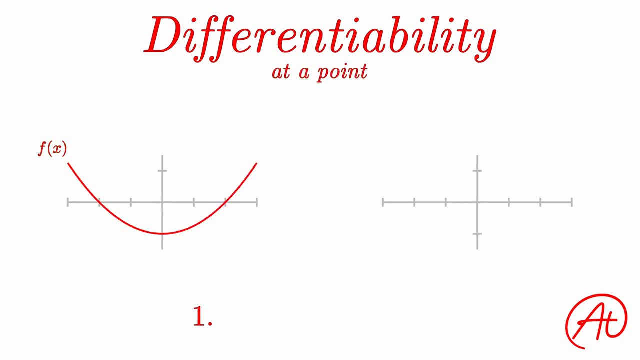 a point. In order for a function to be differentiable at a single point- x equals a- all that we need is for the function's derivative to exist at that point. For this function, its derivative looks like this where it starts at some negative value and steadily increases to some positive. 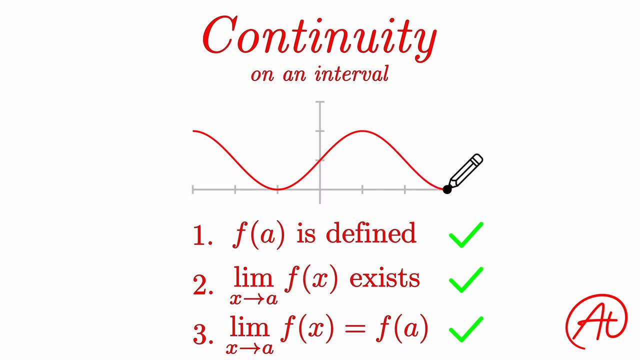 up your pencil, then it is continuous along that interval. So now, using this information, let's take a look at what causes some functions to be discontinuous. In this example, the function is not continuous because there is a hole right here with no other value for that x, so f is not defined for that point. 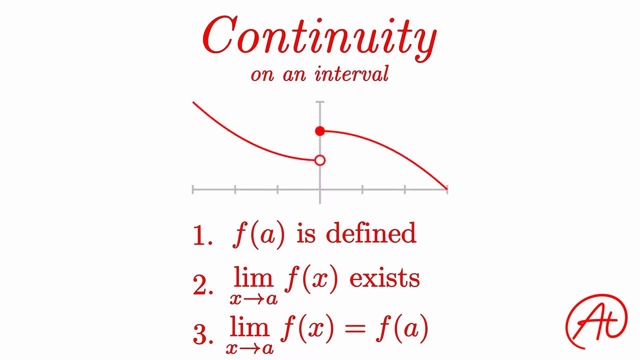 In this example there is another hole at x equals zero, but this time the function does have a value for this x. it's right here, so f is defined. However, for this example, the limit as x approaches zero from the left is this point, but the limit as x approaches. 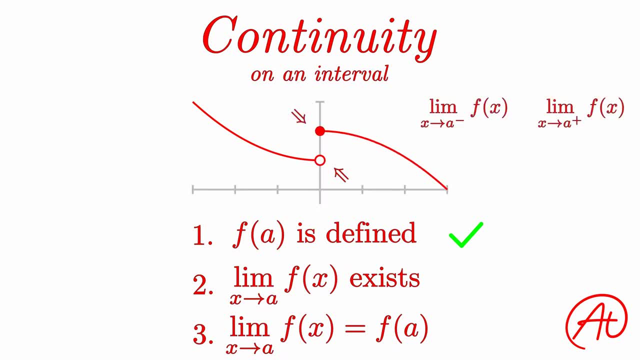 zero from the right is this point. so the two limits are not equal, making the overall limit as x approaches zero not exist. Now for this example. once again, f is defined where the hole in the function is. so we pass the first rule, This time the limit as x. 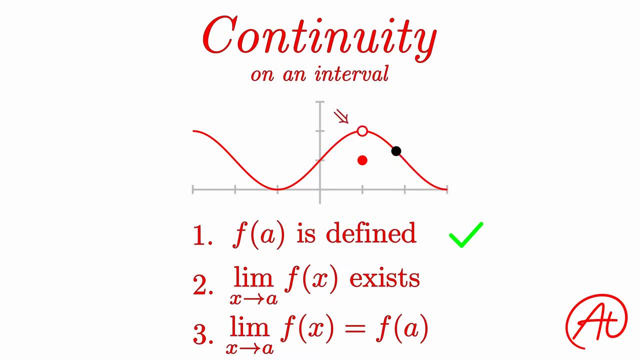 approaches a from the left is here, and the limit as x approaches a from the right is that same value. so the overall limit does exist. However, for this function, the overall value for the limit does not equal the value of f at that point, so this violates the third. 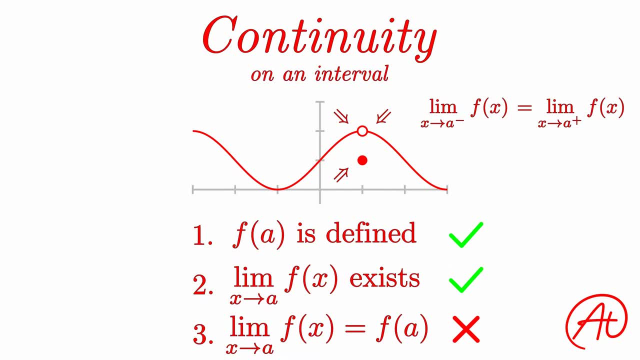 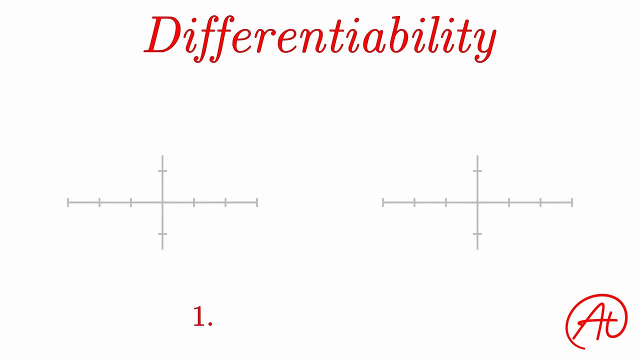 rule and makes the function discontinuous. Okay, now that we went over continuity, let's discuss differentiability. But first, if you're finding this video helpful so far, please smash those like and subscribe buttons to support us. Alright, just like we did for continuity, let's first talk about differentiability at 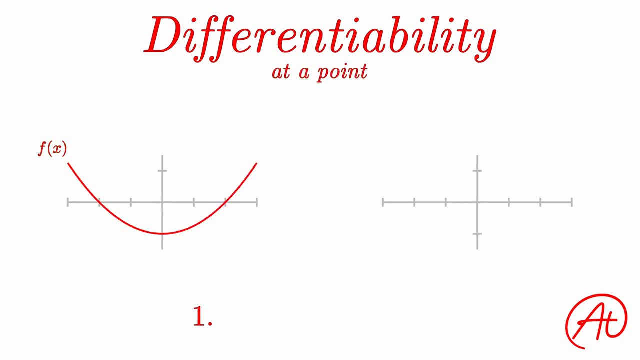 a point. In order for a function to be differentiable at a single point- x equals a- all that we need is for the function's derivative to exist at that point. For this function, its derivative looks like this where it starts at some negative value and steadily increases to some positive. 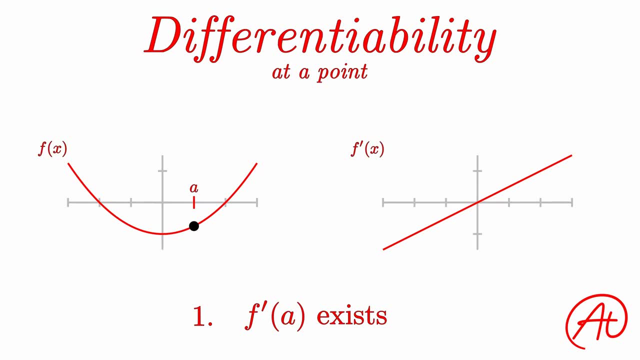 value. So for this graph the derivative absolutely does exist, for x equals a, or in other words, the function has some slope value at x equals a. Now let's talk about what it takes for a function to be differentiable on an interval. 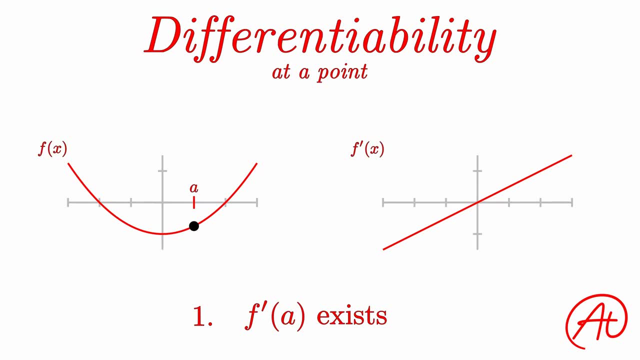 value. So for this graph the derivative absolutely does exist, for x equals a, or in other words, the function has some slope value at x equals a. Now let's talk about what it takes for a function to be differentiable on an interval. 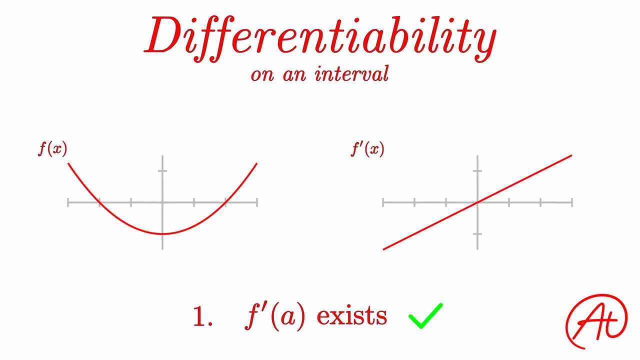 Just like continuity. in order for the function to be differentiable on an interval, the function must be differentiable at every point within that interval, Or in other words, the function's derivative must exist for every point. To help solidify this concept, let's take a look at a couple examples that aren't differentiable. 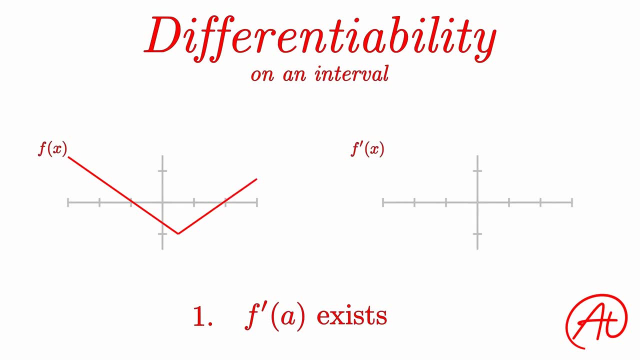 First let's look at this function. For this example, its derivative looks like this: where for the first half of it the function has some negative slope value, Then at this point the slope instantaneously jumps up to some positive slope value and continues for the 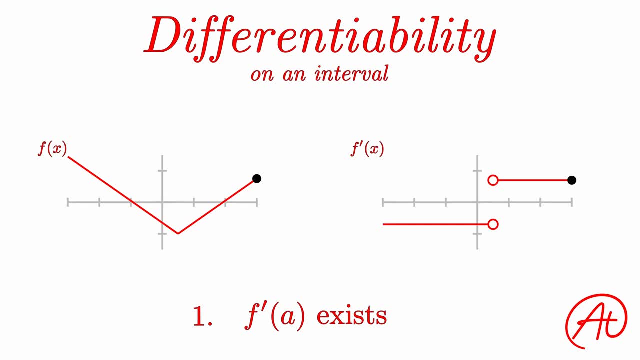 remainder of the interval To the left and right of this corner point. the function is differentiable because its derivative exists. However, right at this point, we don't know what the slope value is, so the entire function is not differentiable on this interval. 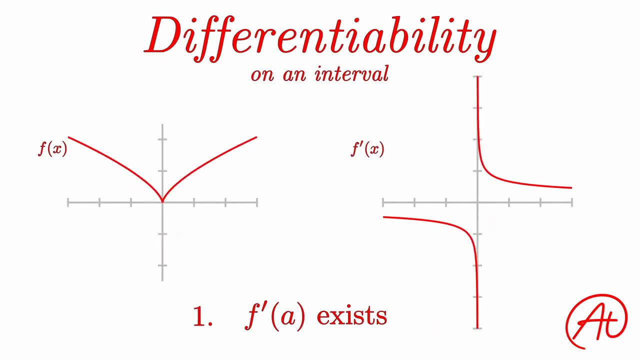 The same concept applies to this type of function. Again, to the left of this cusp point there is some defined negative slope value, and to the right there is some defined positive slope value. But right at the cusp the derivative instantaneously jumps from negative to positive. 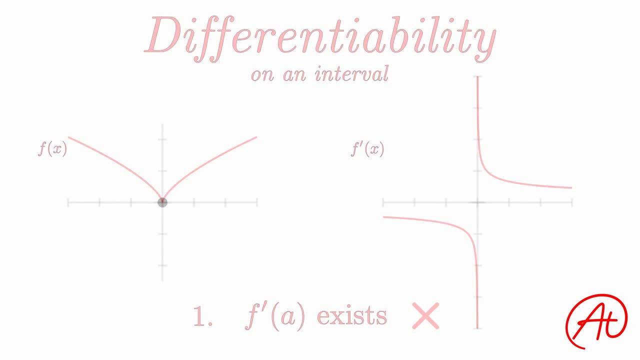 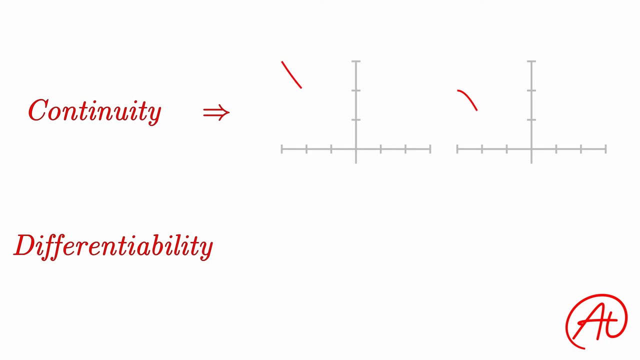 making the entire function non-differentiable. To recap, here are some rules of thumb for remembering continuity and differentiability. In order for a function to be continuous, you must be able to draw the function without picking up your pencil. In order for a function, 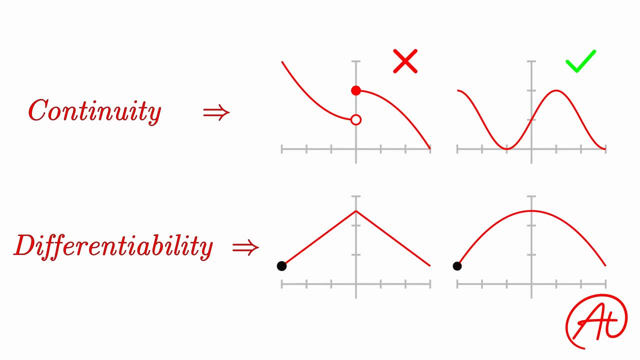 to be differentiable. the function must be smooth, without any sharp points or instantaneous changes in the function's slope. I hope you found this video helpful. Whether you did or didn't, we'd love to hear what you thought we did well or what we could do better down. 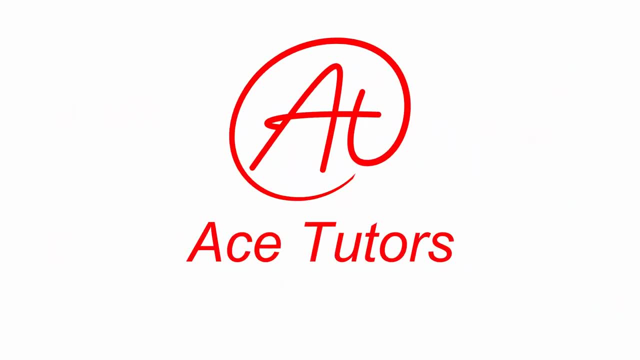 in the comments. Thanks again for watching and remember you have big dreams. don't let a class get in the way. Subtitles by the Amaraorg community.